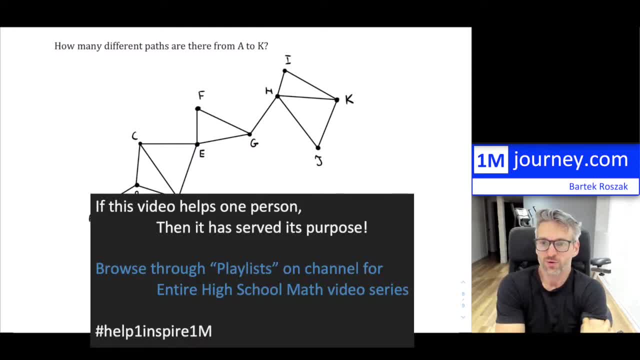 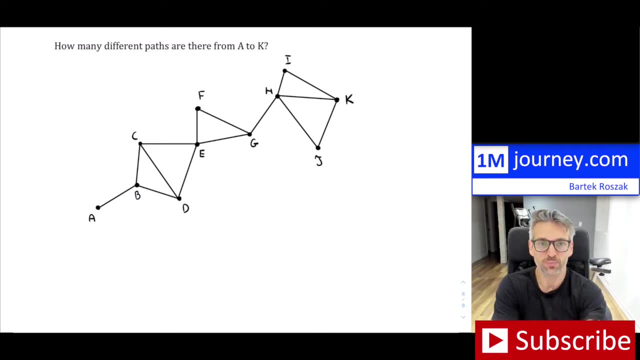 Welcome to this example. So we have this weird figure here and this example actually ties in Pascal's triangle. So what you learn in Pascal's triangle in kind of ordered counting, I'll put up a link up above there to Pascal's triangle and some kind of thought process behind it. So I think 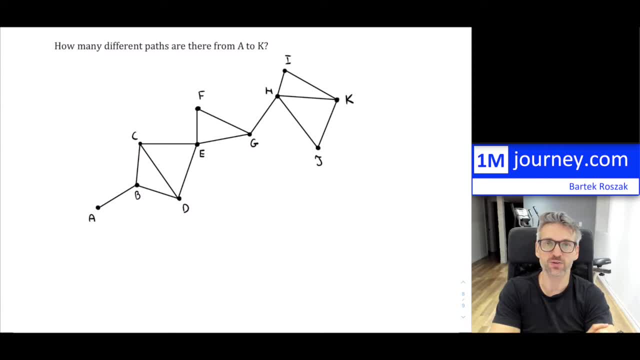 it's very useful because it is used in the application of counting the number of paths. It uses kind of the same concept. So you know when you're doing paths. you can either have- sometimes you'll have- like a checkerboard and you want to see when the checker is going to get to a certain 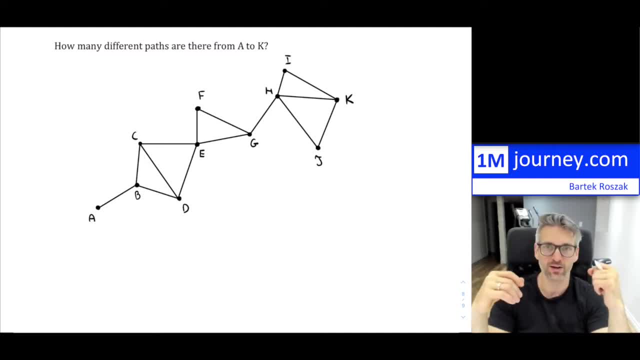 point and how many different ways can they, can it get there? Or you know you have kind of communication links between, maybe, cities and then you know you have all of these communication links between cities and you want to know, okay, well, how many paths are there from one city to another in terms of the communication? So this 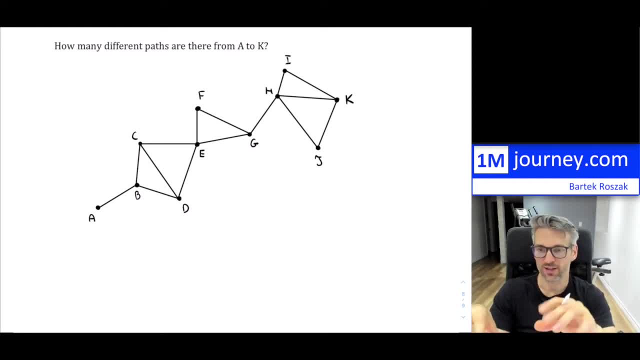 is exactly it. Instead of cities, we have letters, but you can think of, you know, A being a city, B being a city, C and D and so on, And these cities are connected by lines or communication links in some way. They're asking us in this question to go from A all the way to K and find out, okay, how. 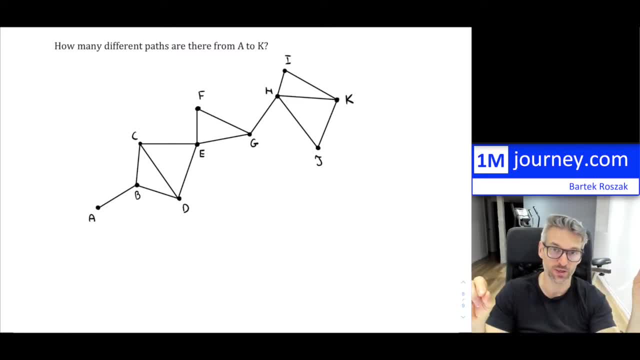 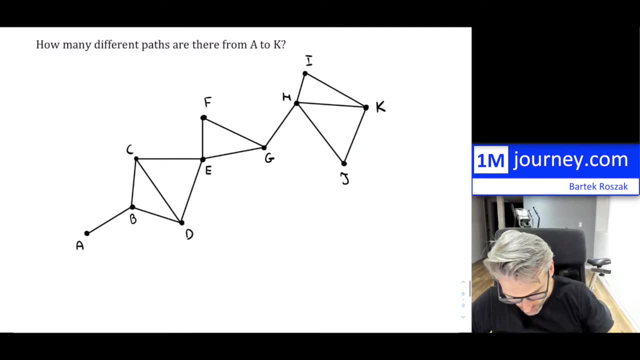 many total paths are there to get from one point to another, So let's do that. So I am going to use the concept of Pascal's triangle in order to do this. So I'm going to be starting from right here and I want to be ending up all the way over here. Now you can draw. 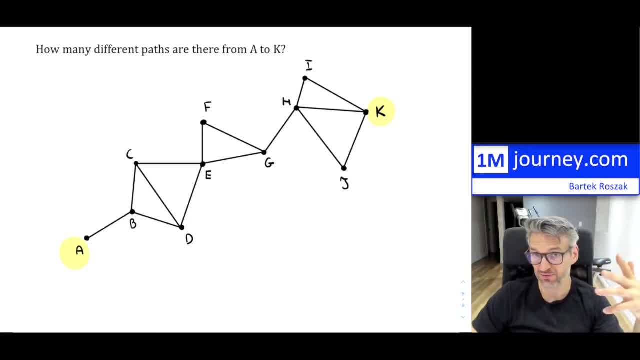 the paths one by one and it would be get it would get annoying and extremely complicated in terms of, you know, overwhelming maybe in terms of looking at the whole thing. So, instead, what we will do is we're going to just create the paths from each city to the other. So we're going to do that. So 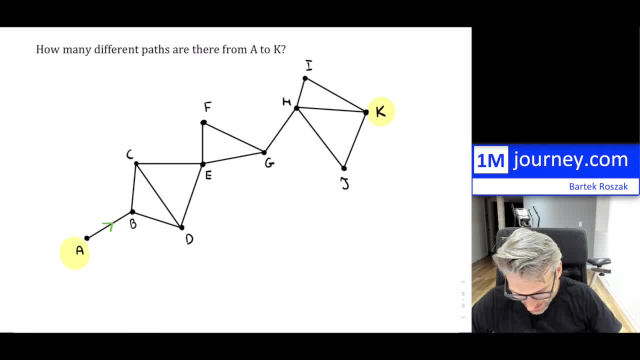 the next. so, for instance, to get from a to b, there's only one way to do it, okay. so i'm going to put a little one there to go in this direction. now to go to c. okay, you will notice that there's only one way from b to get to c. now we're assuming we can't just keep going back between cities, right? 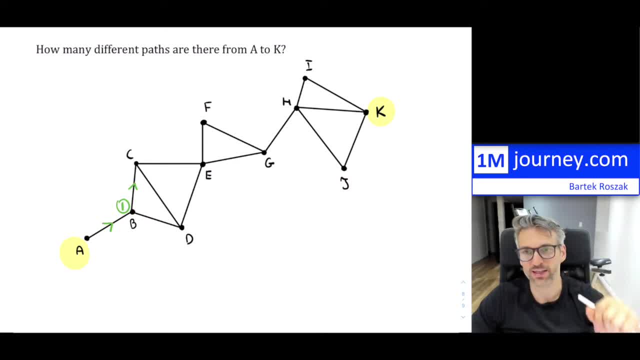 once we traversed something. you know we're not going to be traversing it again, going back and forth, back and forth. so we're kind of, you know, doing the paths which have the least amount- all right, okay- of the direction. so to get to c, there's only one way to get there, um, from b. 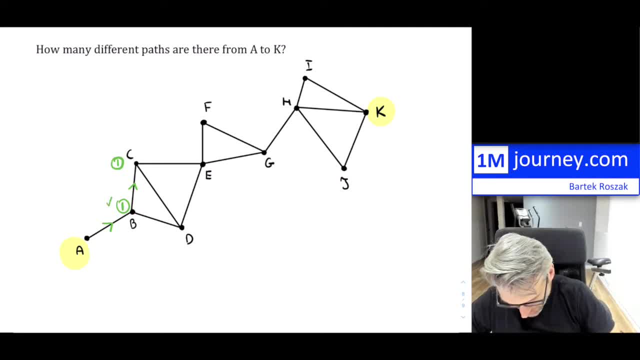 okay. so we're just going to be looking at this, okay, and then doing that answer right here. so now to get from b to d, there's also only one particular way. but now something interesting happens, because you will notice that i can actually go, so i'm going to kind of change. 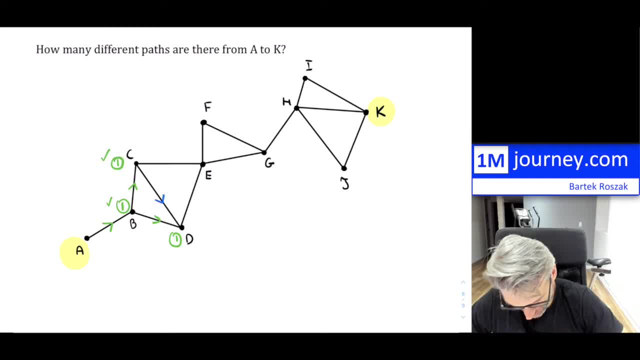 the color here, notice that i can go from c to d. okay, in this direction right now, we know that to get to c there was one way, okay, and now to get to d. so to get to d right here, if it was from b, there was only one way to do it directly. but now, okay if we. 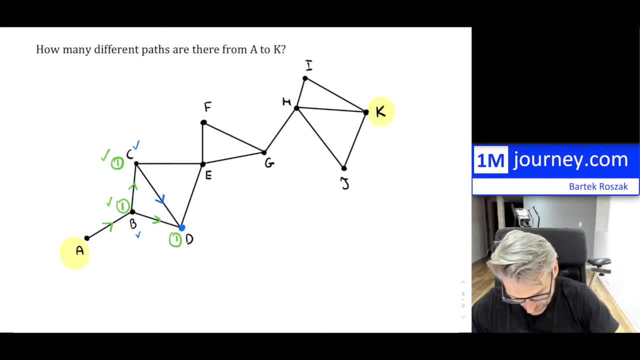 can both from C and from B, then we would say, okay, that's one plus the one. so this is actually two different ways to get to D, and the two different ways would have been the AB okay to D and the ABC to D. so those would have been the two. 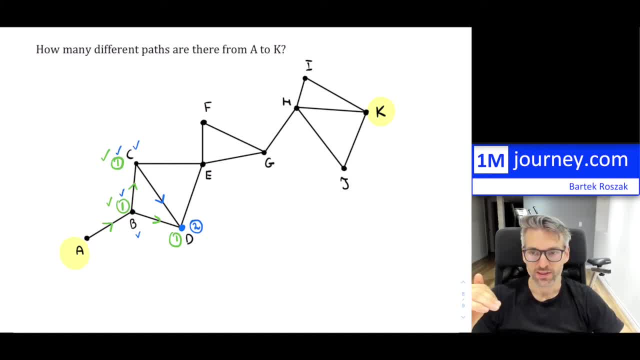 different paths there. all right, so from C, okay, and then from B we can get to D. now you can do that also in the other direction in terms of getting to C, so I can get to C right here, going in this direction, from B, so I can get to C from. 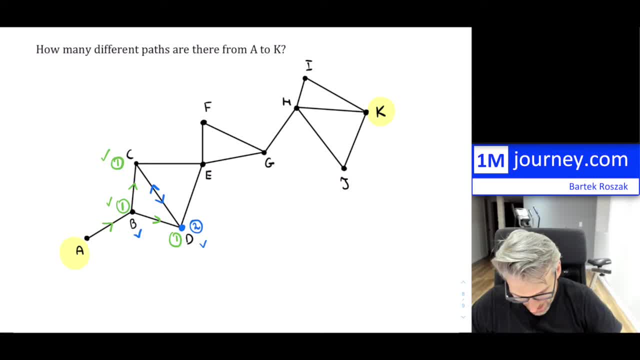 B and from D, and that would have been. so now notice, okay, that going in this now I can't traverse back, so I'm not going to be using this two right here, because I would. I don't want to go back, so I'm going to be using the green, so that's. 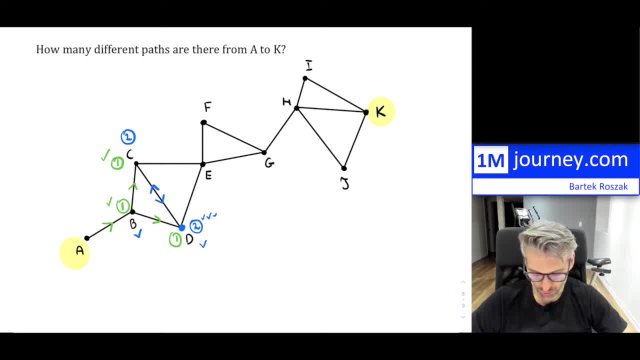 the way I'm going to be using the green. so that's the way I'm going to be using the one plus the one. so this would have been two ways to get to C. all right, and that's something you're gonna have to think about a little bit. okay, now I'm 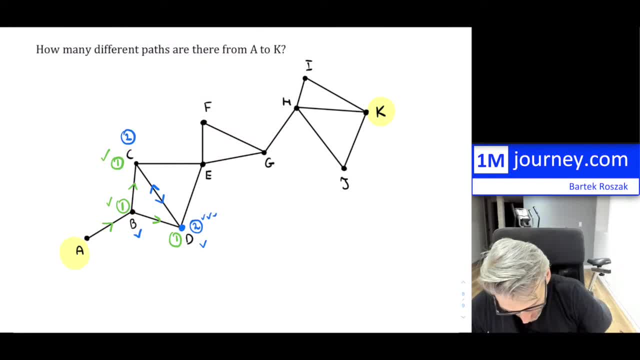 gonna go back, okay, and now we continue. so now to get to E. so I can get to E from C and from D and notice there's two ways to get to C and then two ways to get to D. if I count all the paths, so that's two plus the two, so that means four. 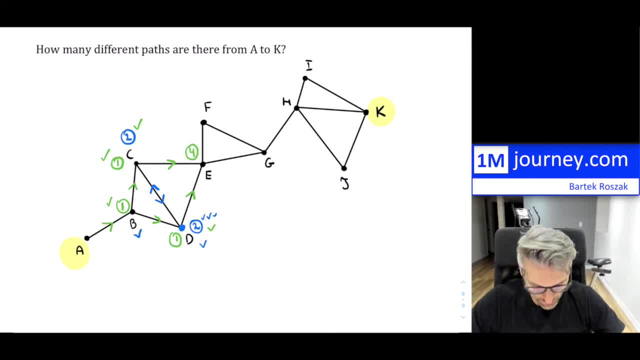 total ways to get to C and then two ways to get to D. if I count all the paths, so that means four total ways to get to E and now to get to F. okay, so that there's only one way. okay, so that would have been just four. okay, that's in this. 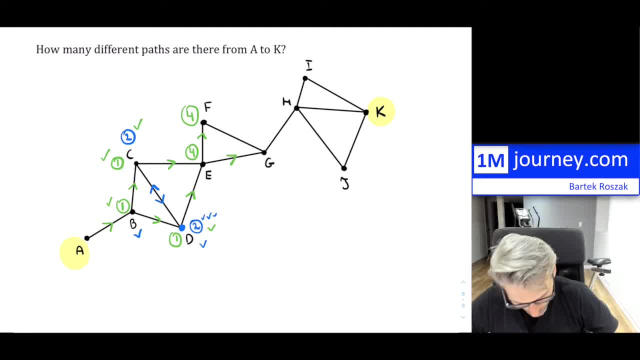 direction and then that's going in this direction. so that's from E to G. so this is also four, right, because it's for this. but it's also going through F, so I have to add up the two nodes there. so I'm going to be adding this and this. so now, 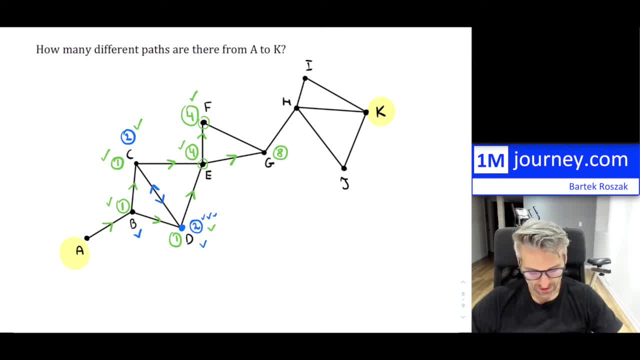 this is gonna give me eight, and now I can continue. so now there's only one way to get to eight- sorry, to get to H. and now we eight different ways, because I'm just looking at the previous node and now again. so now I'm gonna be running. 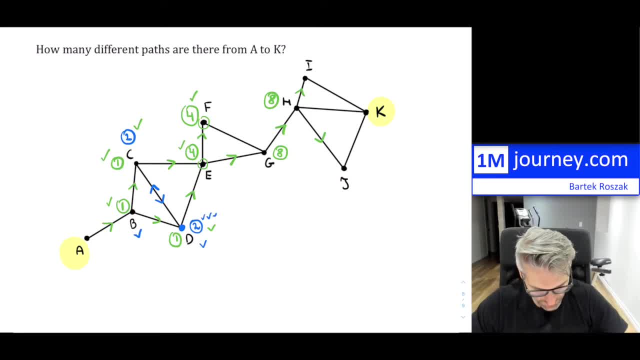 into problems. okay, so right here, notice that what I have is to get to J, so there will be eight different ways, right from H to get to I. there's eight different ways To get from H to K. okay, there's eight different ways, right. 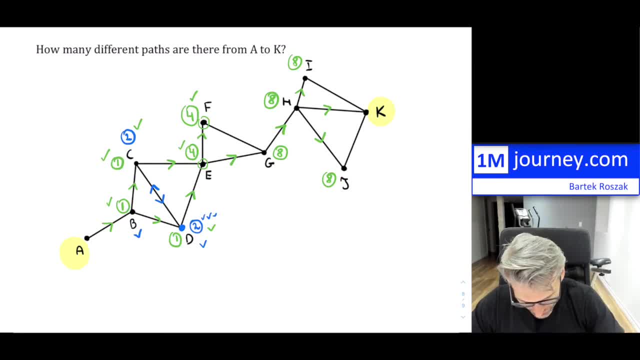 However, okay, now notice that you can also get to K from here. So that would have been eight okay going from J, eight okay going from H, and then eight going from I. So in total, so that's eight plus eight plus eight, which is 24 different ways that we would have there. 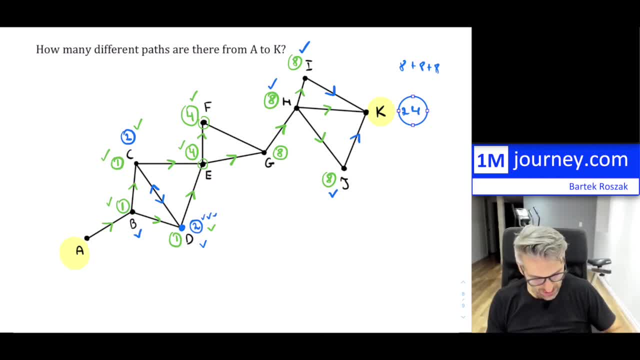 okay. So that's an interesting example, to be able to use Pascal's triangle in order to actually count the number of paths, And I would encourage you, you know, to kind of erase this and then do it on your own And, in particular, you know understand what has happened around here.